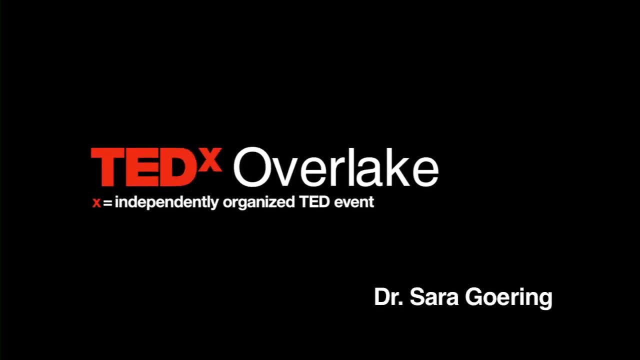 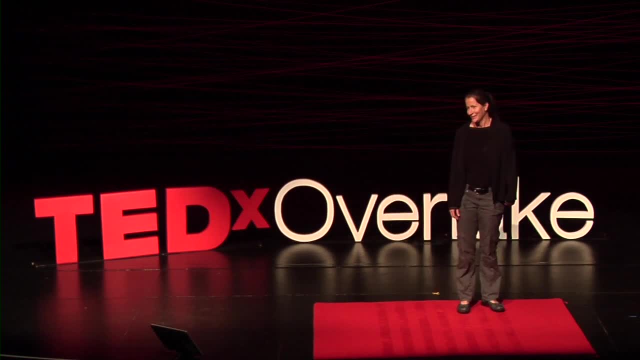 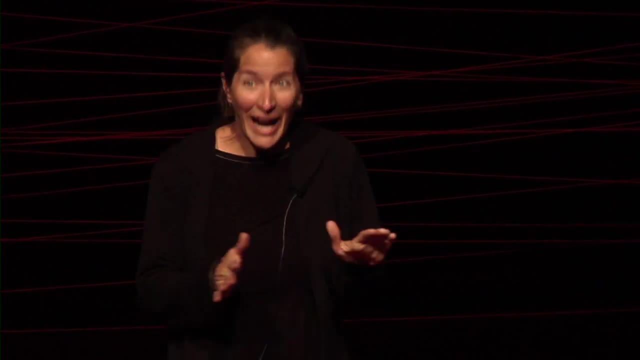 When I tell people that I'm a philosopher, casual conversation, I typically get a look, And it's a look that I think is a bit of a mixture between awe and fear, As in: wow, really cool stuff, Deep questions And also- oh my God, please don't make me defend everything. 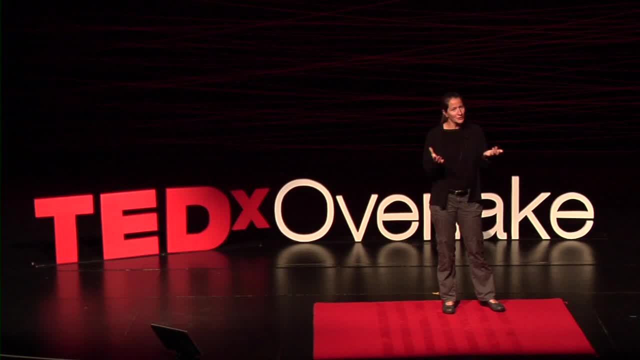 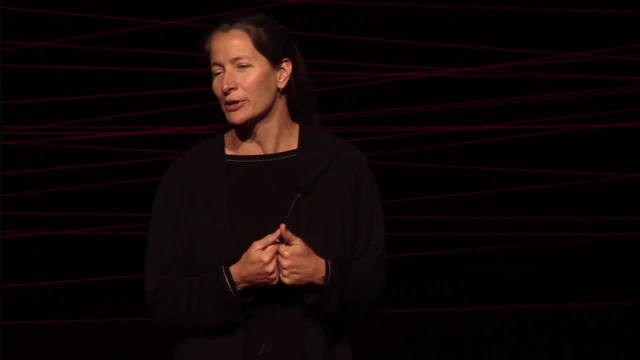 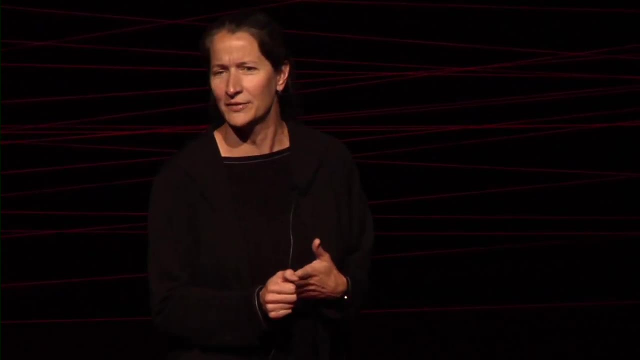 I think I know. So philosophy is really something that when I say I teach philosophy to kids as well as adults, those same people look at me like I might be crazy. Philosophy is understood to be a deep, abstract, rigorous, difficult kind of discipline. People don't. 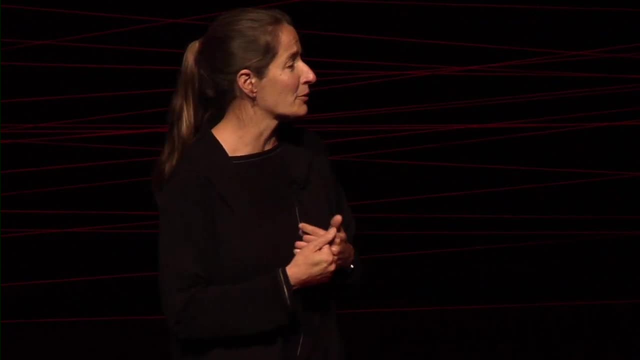 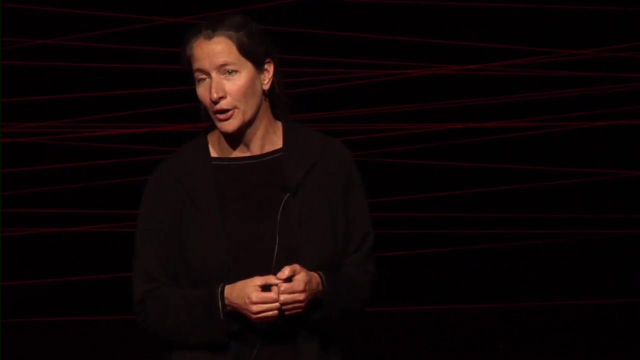 think that children are capable of doing it. When they look at me like I'm crazy for doing it, I think you're wrong. Kids are actually very natural philosophers. They ask these kinds of questions on their own, And it's our job to help give them uptake on those questions. So what are philosophical? 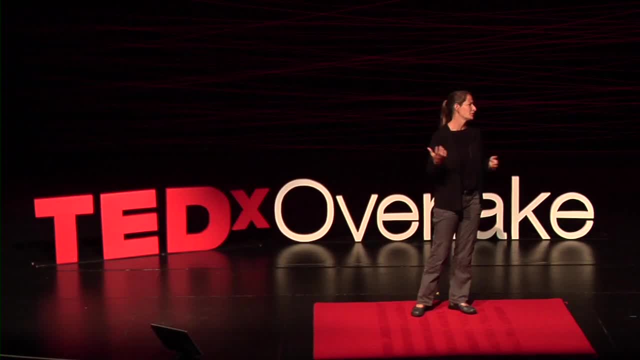 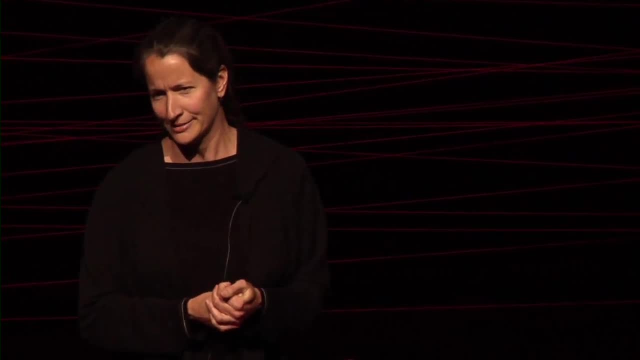 questions Right, Philosophers are wondering all the time, from the ancient Greeks through today, all about the nature of the universe and our place in it. Philosophers want to know, for instance, if we're really free And what it would mean for us to say that. 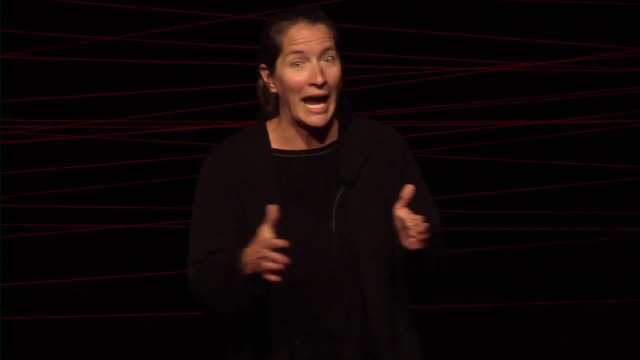 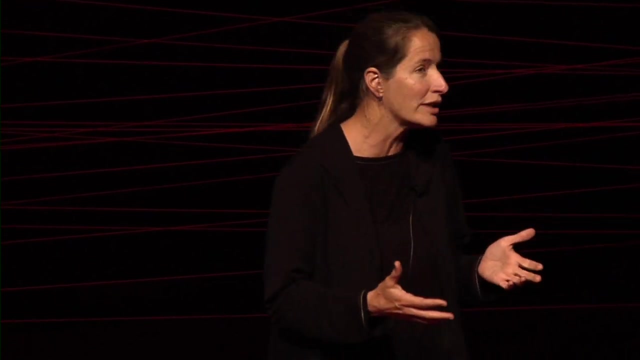 we're free. And could we both be determined and free? Most people think that's absolutely insane, impossible, Right, But a lot of philosophers believe that that's the only way we can be free: if we're both determined and free, Or we'll ask questions about the nature of. 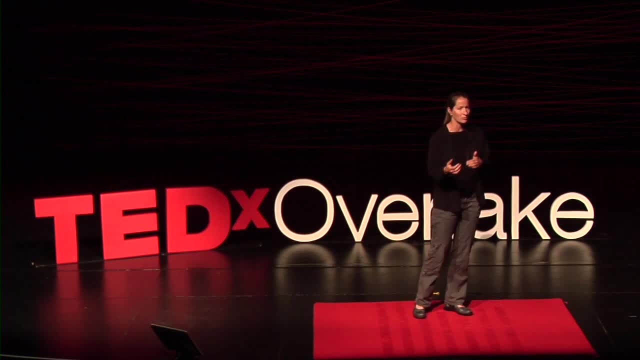 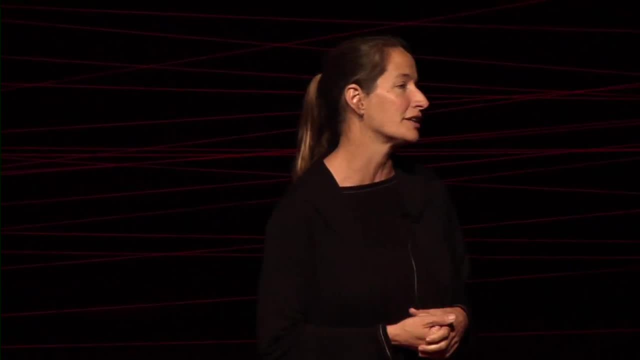 right and wrong? Right, We don't just want to know the answers- what's right and what's wrong, what should I do, what should I not do- but the reasons behind that and whether we're really justified in thinking that certain things are right and wrong. We'll also ask: 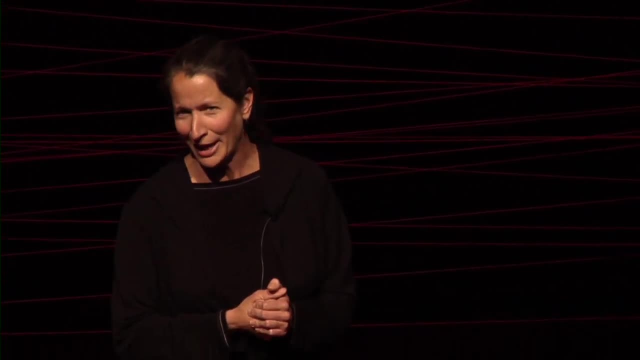 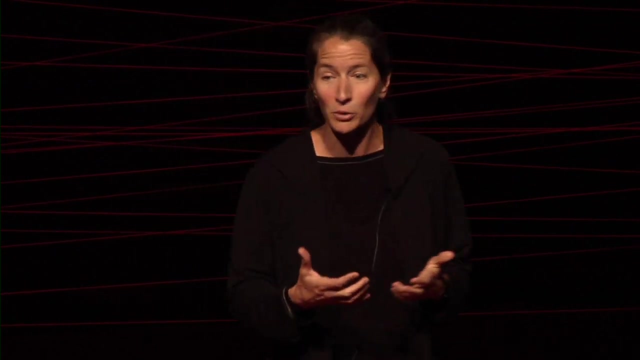 right. if the sun's going to burn out in five billion years, does anything really matter? How would we know if it does? How do we make meaning in our lives, knowing that we're all going to die, Right? These are the kinds of philosophical questions. 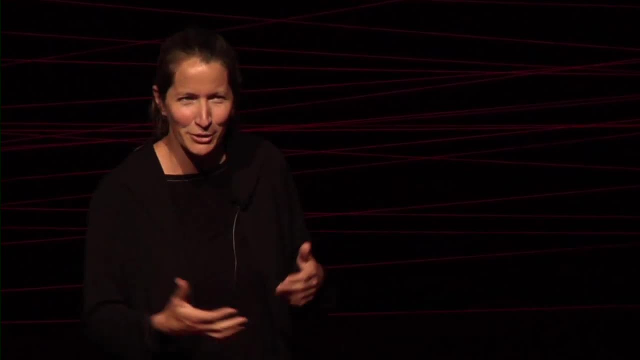 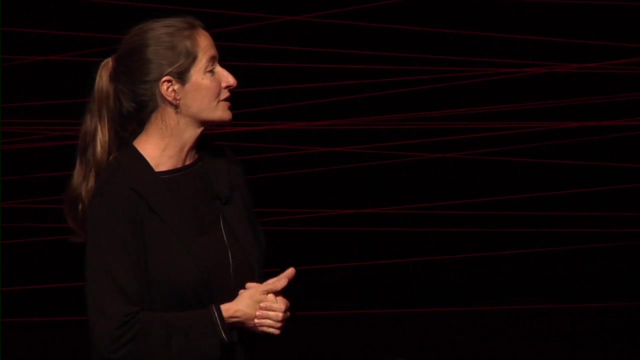 And can you know right now that you're not dreaming? We'll get you to worry about that question. You won't be sure. right after an introduction to philosophy. So these are the kinds of questions that philosophers ask And, like I said, I think kids ask them very. 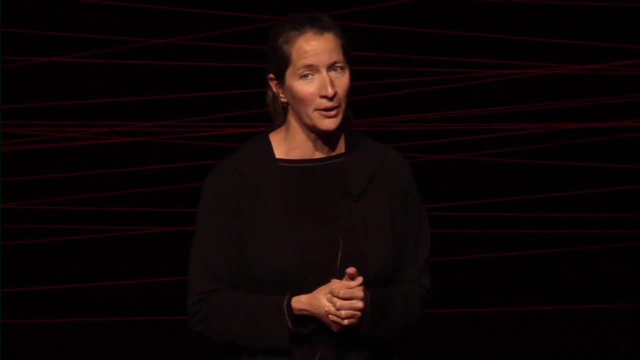 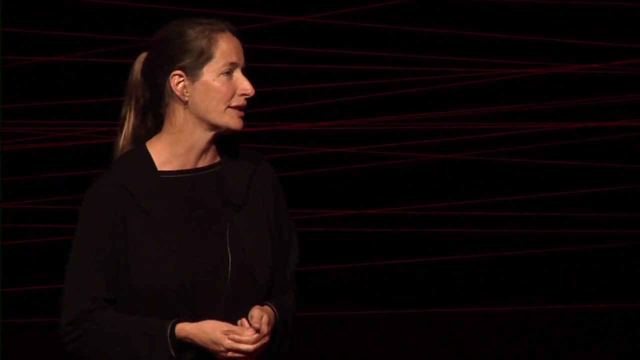 naturally, Adults have a much harder time asking them, in part, I think, because philosophers examine the most fundamental assumptions that we have about our place in the universe and who we are, And it's hard to give those up when we've put them in our background And 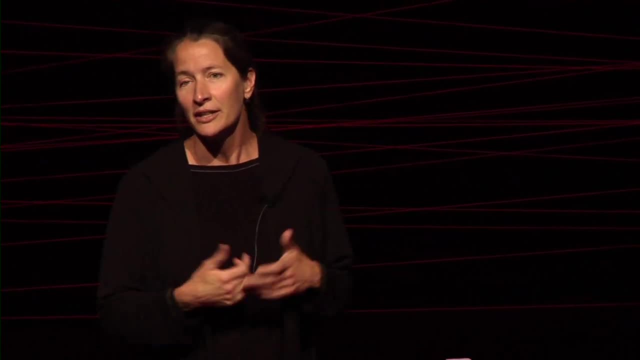 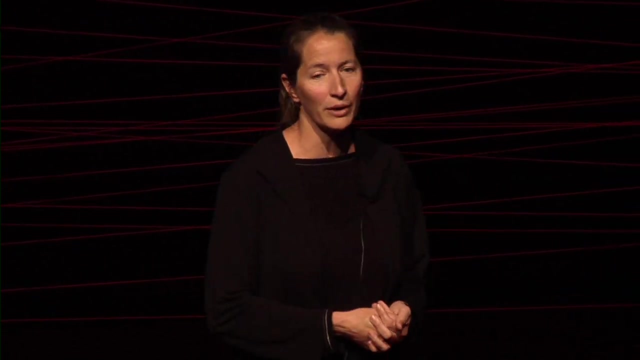 it's hard to echo that, And so what they've found as adults is just like Jim Coposino said earlier: adults have to unlearn those assumptions right, Learn to sort of be aware of what they are and then examine them really carefully, Whereas children are fresh to the 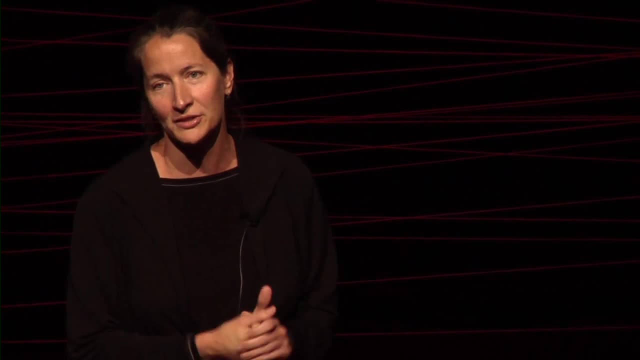 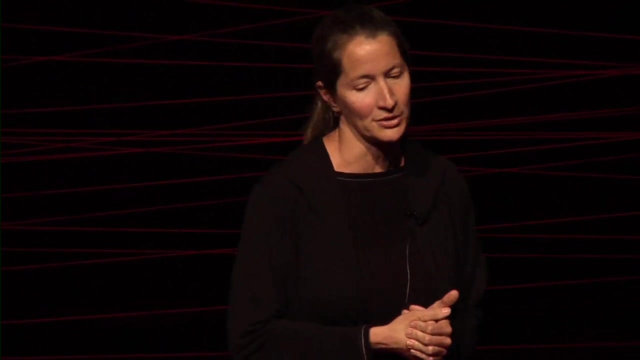 world. They're wondering about where they are and how the world works and what their place is in it. They haven't yet made those assumptions, And so they're very eager and open to thinking philosophically about ideas. So children raise these philosophical questions. 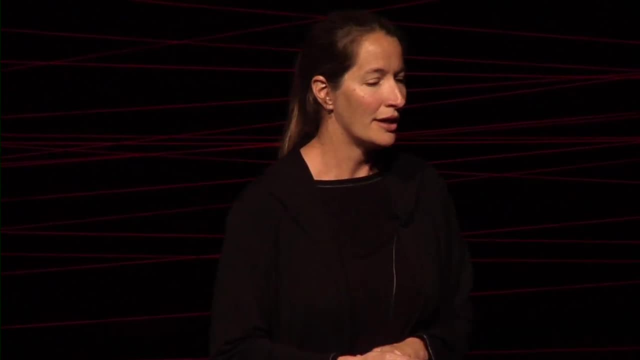 Right, Right, Yeah, Absolutely Yeah, Right, Yeah, Yeah, Right, Yeah, Yeah, Right. through 12th grade and high school, A particular class. I went to a fifth grade and I did a little intro on what philosophy is. 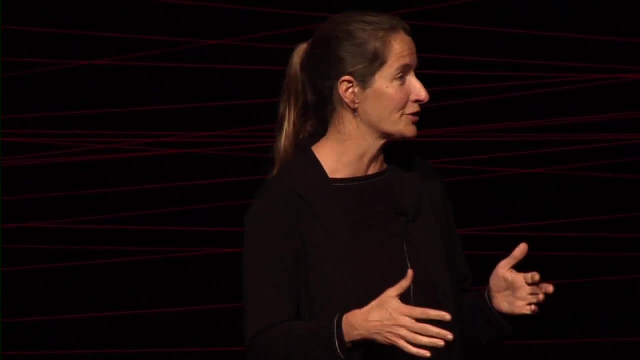 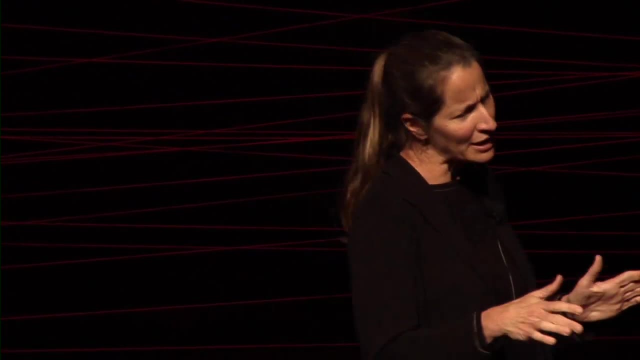 because most people, unfortunately, have never heard of it until they get to college. if they stumble upon a class- And I asked the fifth graders after saying something about what a philosophy question is- just take a minute and reflect and write down philosophical questions. 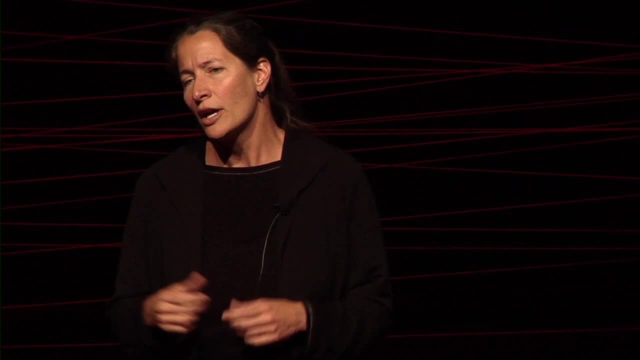 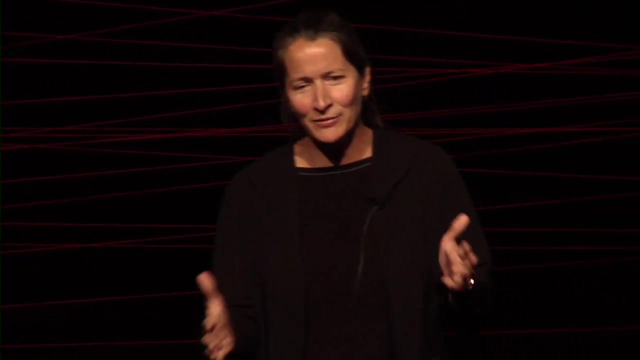 that you ask yourself that you've raised for yourself late at night, when things are calm and quiet, or on a car trip, when your damn DVD player breaks down right, And you have to actually think for a little bit. What are the questions that you ask yourself? 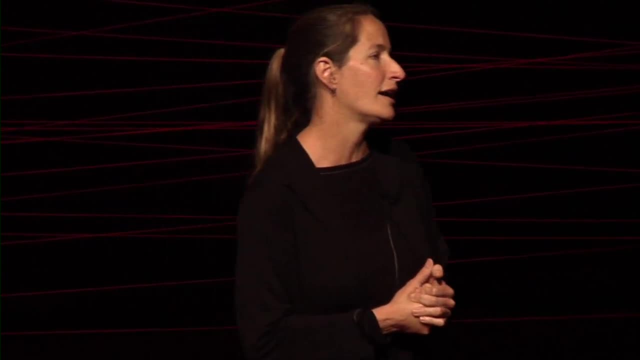 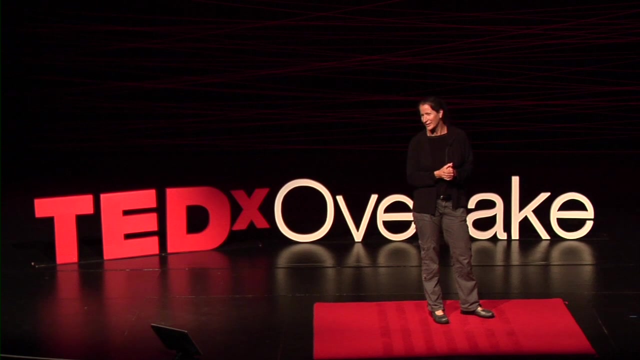 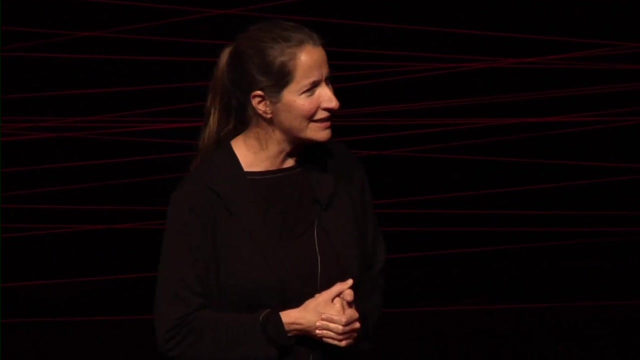 And it's amazing what they come up with. So this particular fifth grade class. some of the questions they asked were: what are numbers And where do they come from? And how is it possible that they go on forever? Or they ask: why do people hate each other? 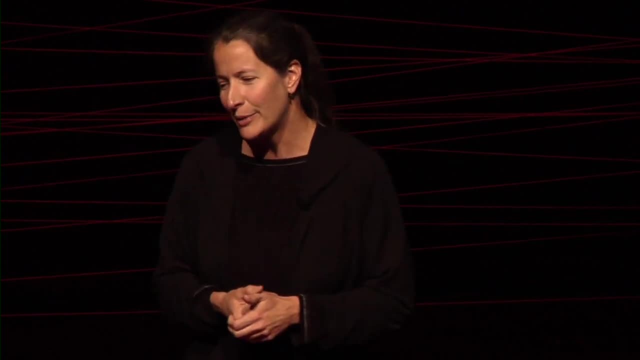 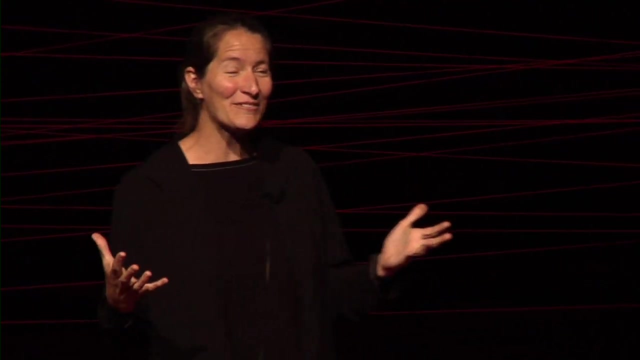 And why do we start wars? And other ones of them ask in a public school if there is a God, who created God? right, These are great philosophical questions. They're questions that deserve a little uptake from the adult world, right. 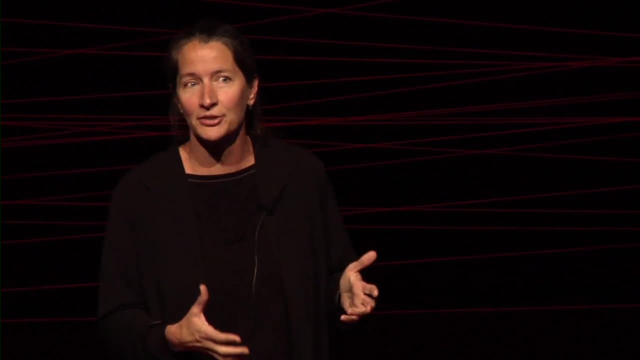 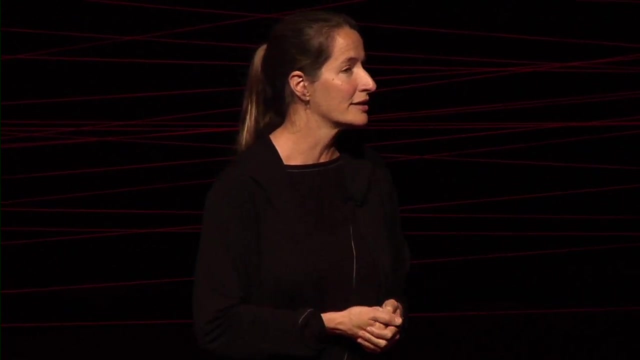 We need to engage kids on the questions that they have. They're trying to understand their world and make meaning in it, And I think, unfortunately, that in our current system those questions aren't getting uptake, So they don't really get uptake in the educational system. 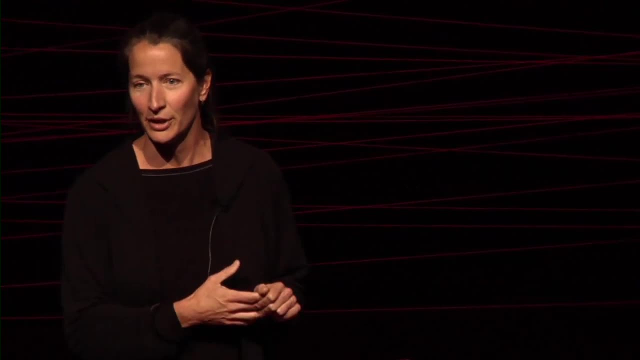 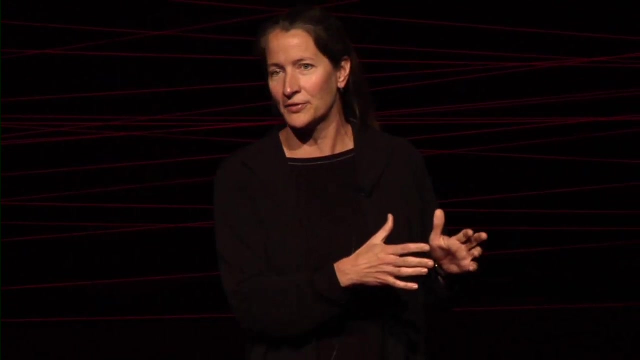 in part because teachers aren't really trained to deal with those kinds of questions. right, The answers are. they're ambiguous. there are better and worse answers, but there's not one clear, right one. You can't teach that for the test very easily. 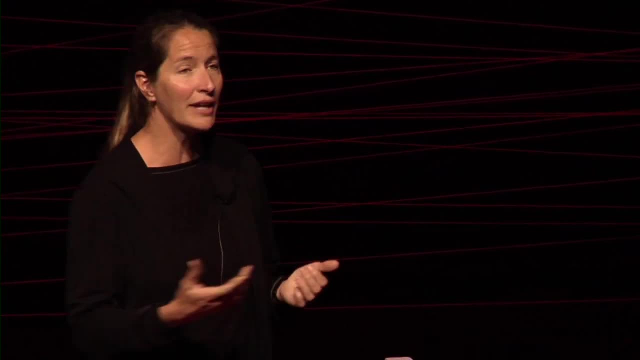 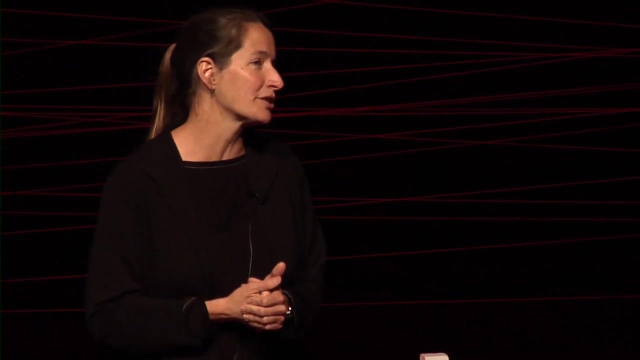 We're increasingly getting funneled in that direction in education. But even at home I think often they don't get uptake Because parents- many of us right- haven't fully thought through these questions and informed our own answers or figured out whether or not. 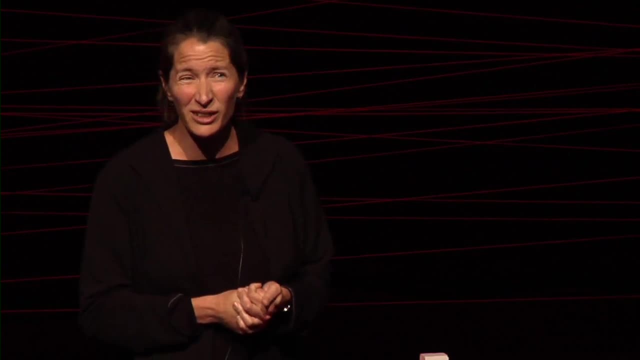 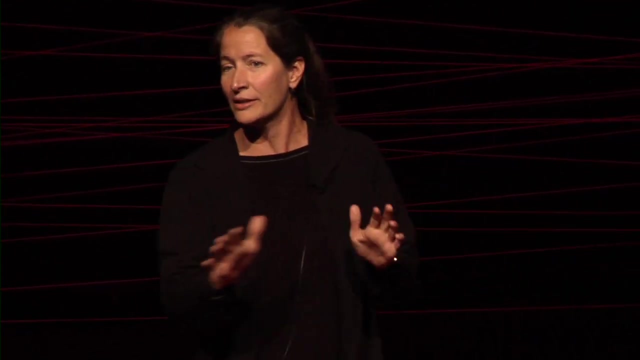 we're justified in what we tend to think might be right about those questions. We're a little embarrassed by that when our kids call us on it And so we fumble right And we maybe put it off a little bit and we don't actually address them. 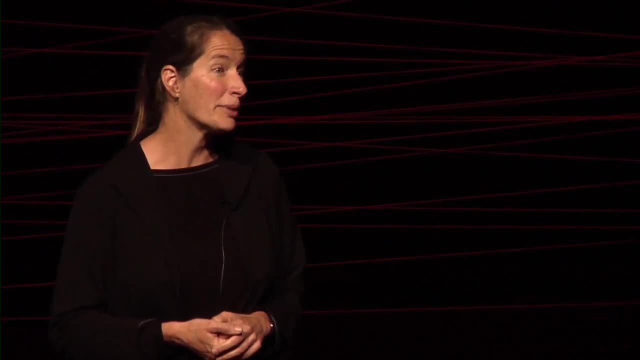 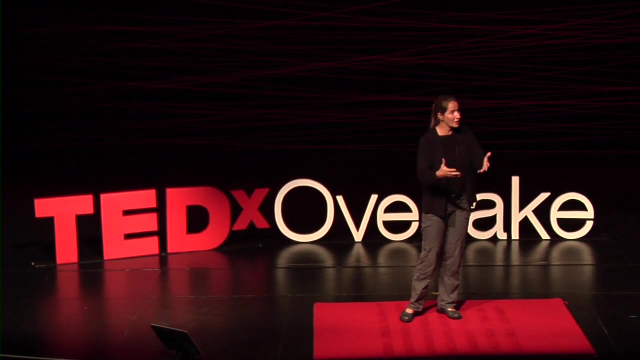 And the result is that kids think these are questions that don't matter. But they do matter, right? They matter for our understanding of ourselves and our place in the world, And so, in the work that I'm doing, we're trying to get philosophy into the schools as a way. 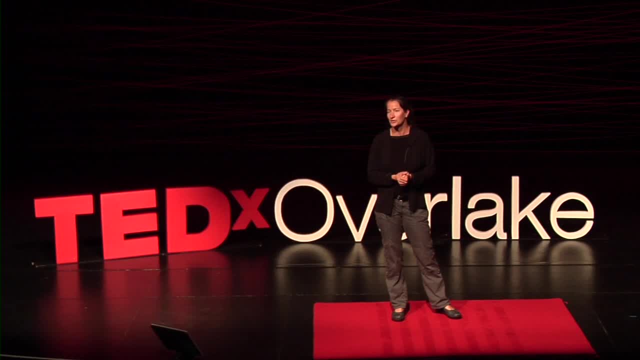 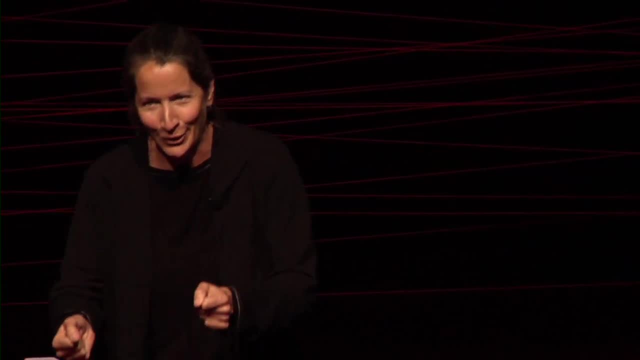 to excite kids about their learning and to give meaning to these questions that they're already raising. So how do we do that We don't take in Kant and Descartes and Hegel and Heidegger and say: read this, Now let's do a little reading comprehension. 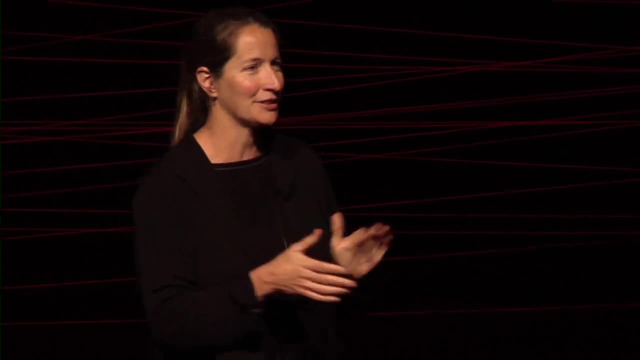 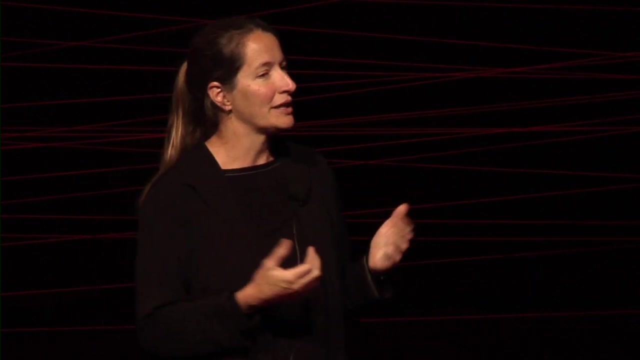 and see what you think You know. of course they would hate philosophy, right Rightfully so, probably at that age. Instead, we go in with the classic techniques from the history of philosophy. So what are philosophers known for? 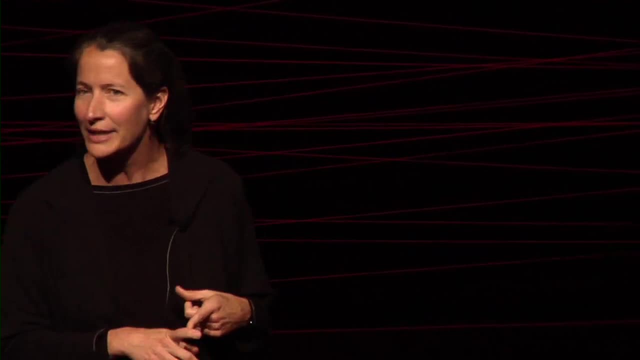 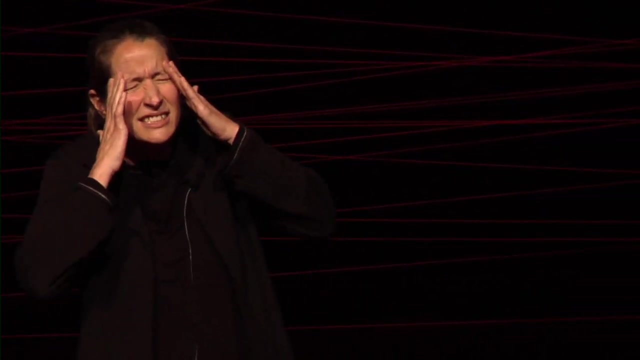 Thought experiments, And the beautiful thing about thought experiments is they don't take any lab space. We don't need beakers, We don't need chemicals. There's no safety training, It's this Right. You have to think really carefully about some hypothetical that we're going to pose to you. 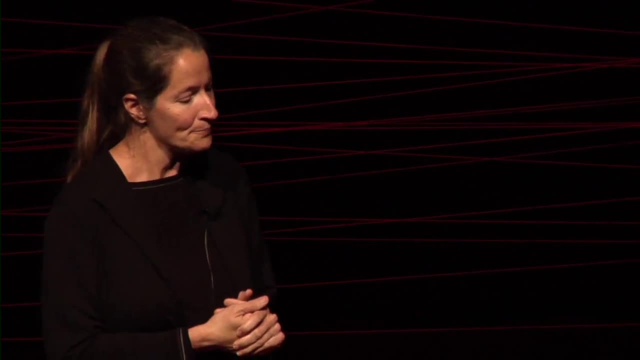 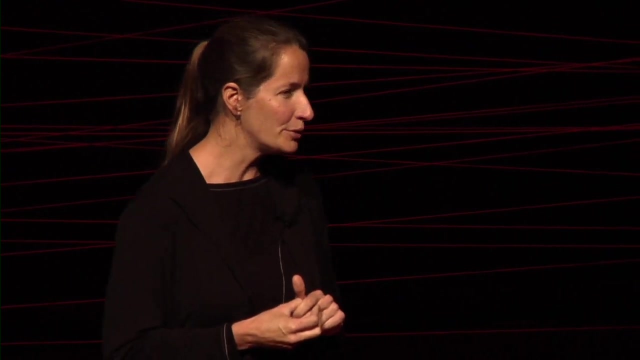 So a famous one from ancient Greek philosophy is the Ring of Gyges. Imagine that you find a ring And if you twist that ring it makes you invisible. What would you do with that ring? We give them a little time to explore that. 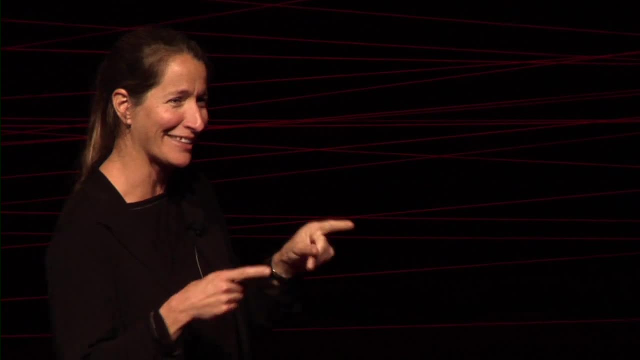 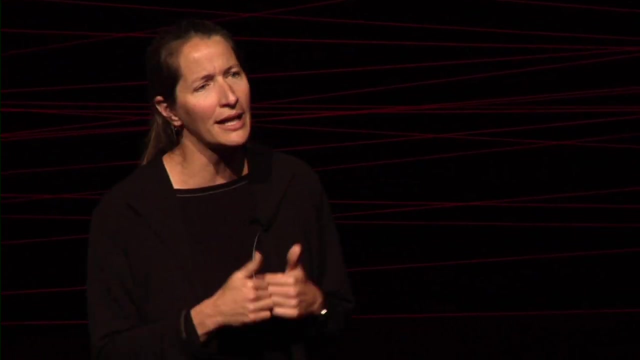 Why would you do that with that ring? And you can imagine the things that they're saying And then, once we figure out why they would do it, why do you not do those things when you don't have the ring? What stops you? 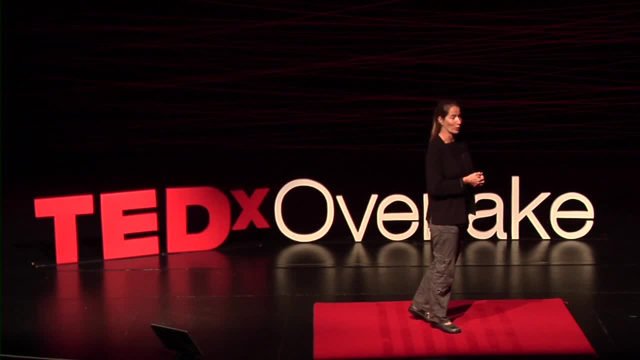 So a lot of them want to do things that are, strictly speaking, wrong, Immoral, Or at least funny and inappropriate. They want to spy on people, that kind of thing. So why do you not do that? What makes those kinds of things wrong? 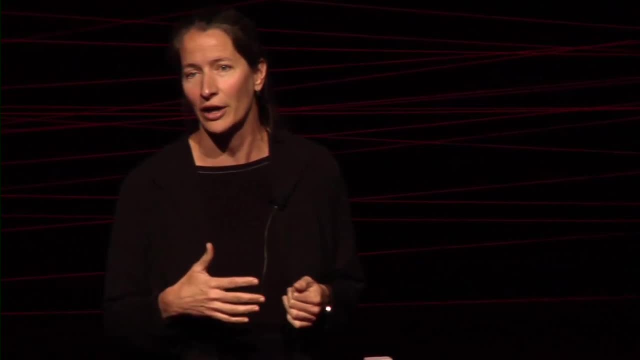 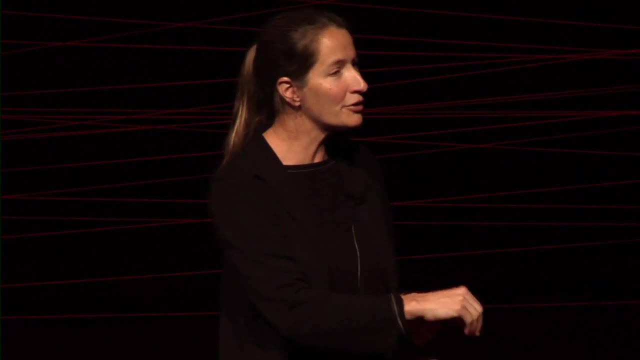 And initially some kids will think: well, what makes it wrong is that we get punished for it. But then we can help them through the process of discussion, come to see that we punish those things because they're wrong. They're not wrong because they're punished. 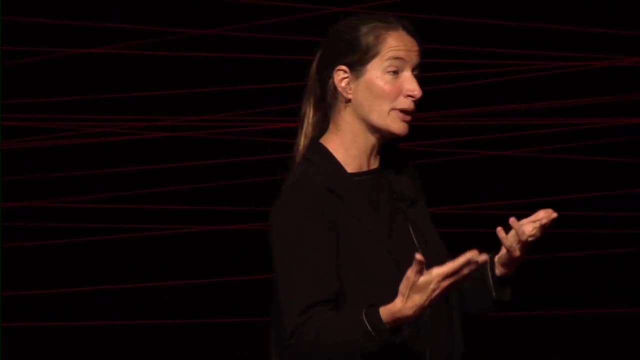 We have to get the arrow going in the right direction And we can build these really interesting deep conversations with kids based on, maybe, some of the things that we've done in the past, based on, maybe, thought experiments that we start with. 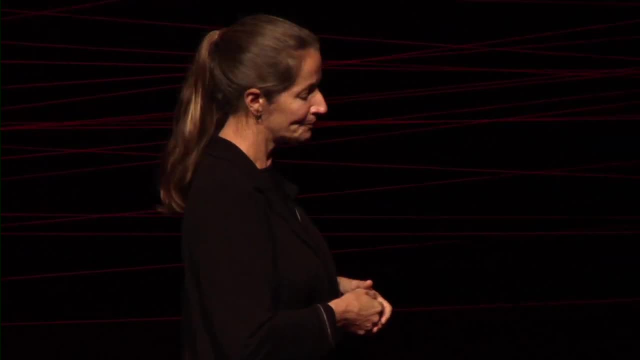 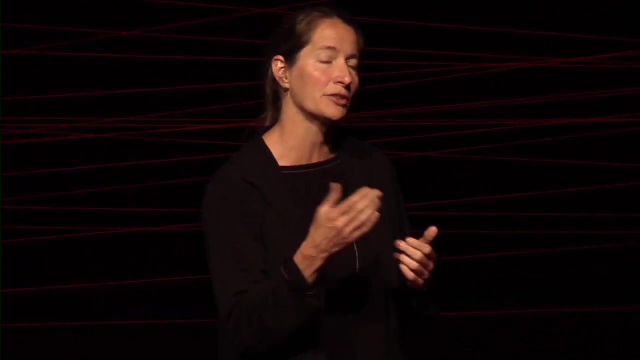 But they're really coming from the kids' own questions that they're raising, Or we'll use philosophical puzzles. The Ship of Theseus is another famous example from ancient philosophy. Imagine you have a boat Over the course of time, maybe five years. 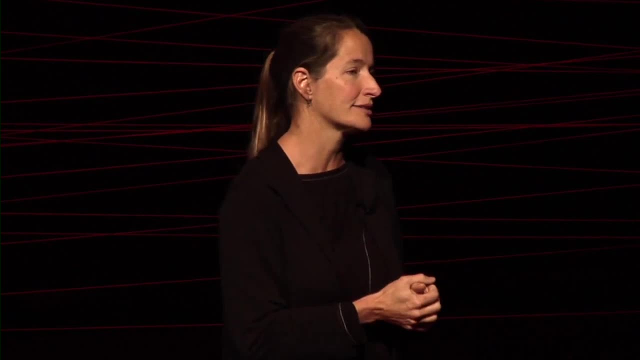 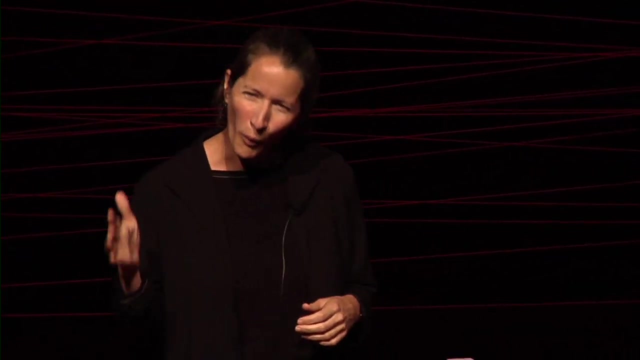 you actually replace every single board or every single part of the boat. At the end of that process, do you still have the same boat Right? Some people's intuition says, yeah, it's the same boat. If you think it is the same boat, why? 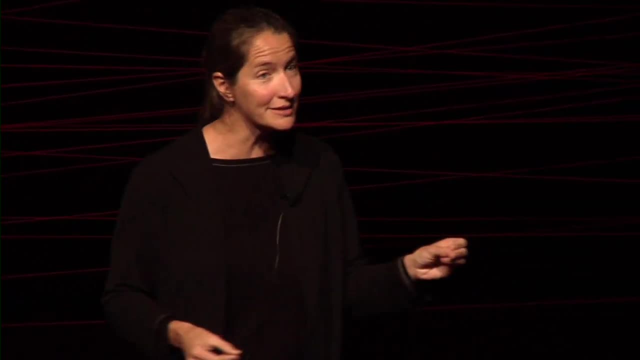 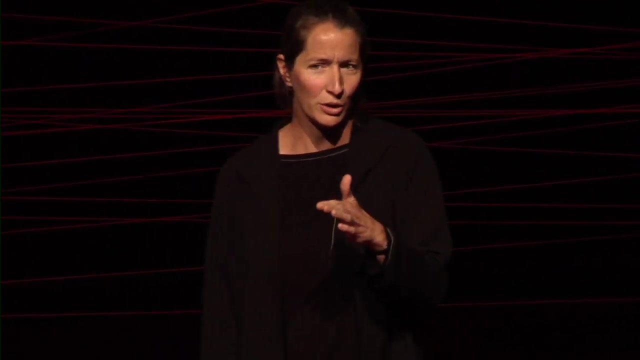 Through that process of change over time. And if you think it's not the same boat, well now tell me, when did it not become the same boat? At what point in this process of change would you have said: ah, now you have a new boat. 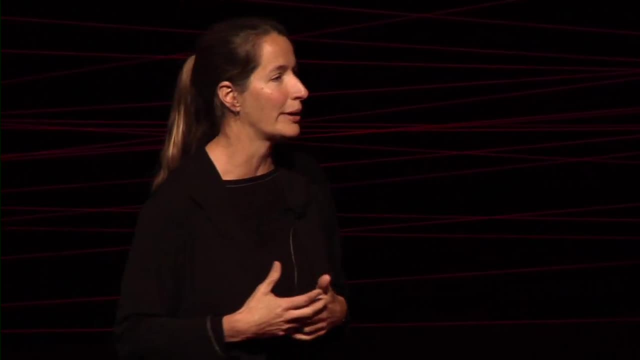 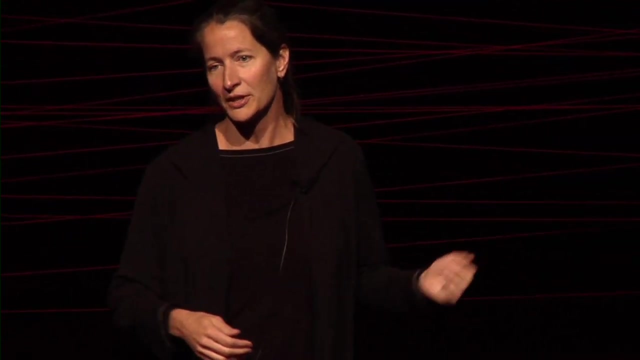 And then starting with the boat, then we can translate that into a discussion about personal identity, human identity. We're creatures who change over time. Are we really the same as our earlier selves? Will we be the same as our future selves? 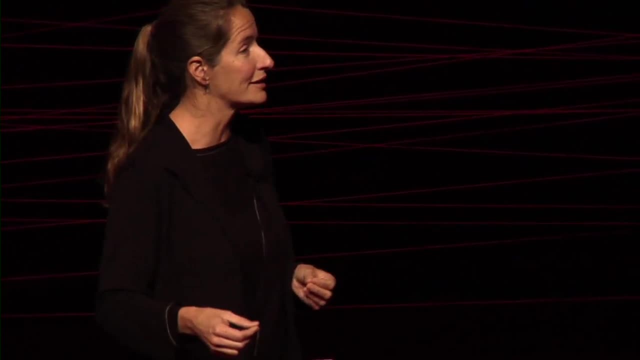 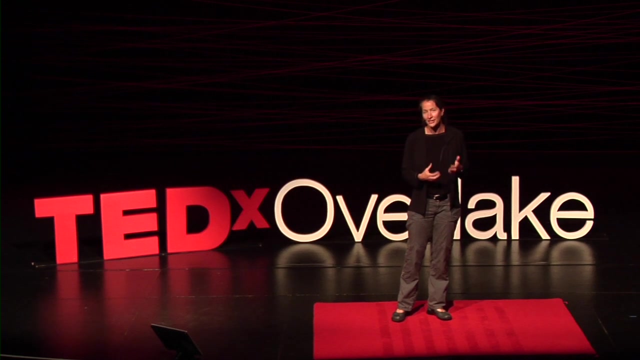 And what allows us to make that kind of claim? What Either Are our brains the same Or how do we retain an identity over all of this change? And the kids love doing this kind of work. They're really interested and invested in these questions. 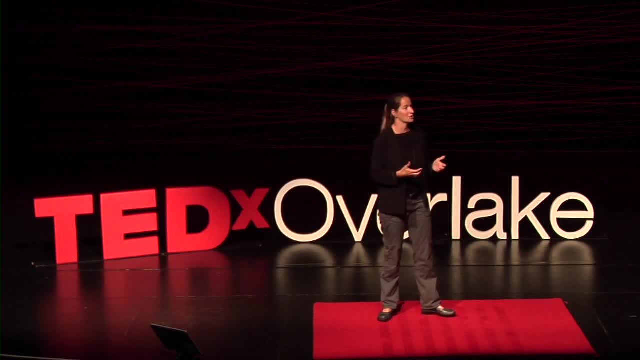 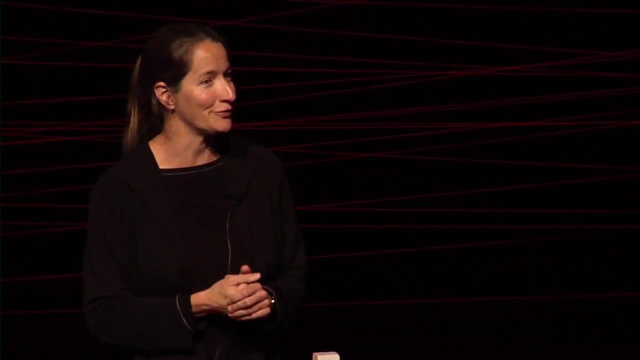 We'll also use just great children's literature. The best children's literature has deep philosophical questions in it. So we'll use even simple things like Arnold Lobel's Frog and Toad Adventures. If you're a parent, you know those well. 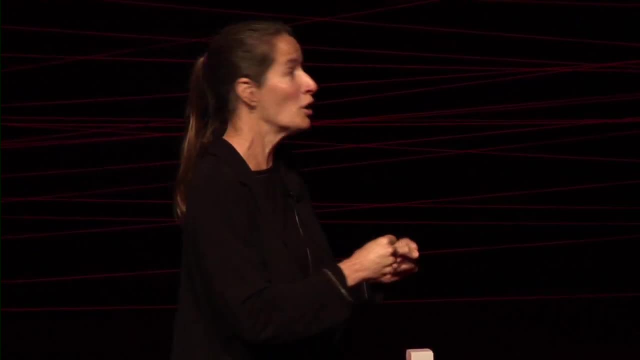 We'll talk about bravery. Frog and Toad run away from a lot of things all the time saying, woo, we're very brave, Look at us run away from the snake- We're being very brave. So we have an interesting discussion with the kids. 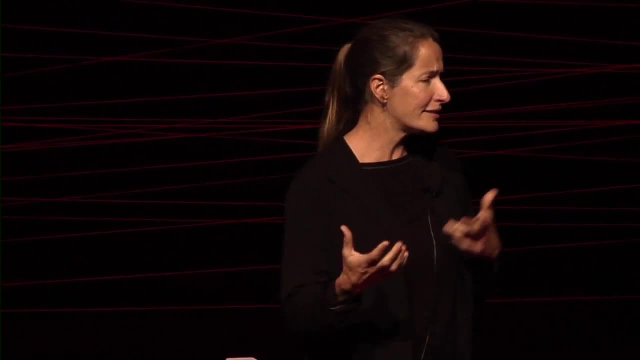 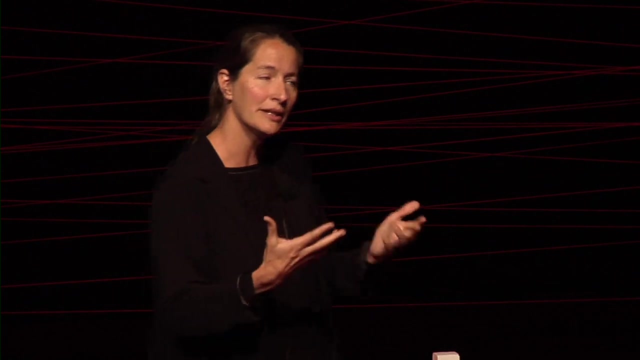 What is bravery? What's the nature of that thing, And can it be in tandem with really being afraid? Is it standing up in the face of your own fear and doing something? So we develop these really interesting discussions out of literature, out of puzzles, out of thought. 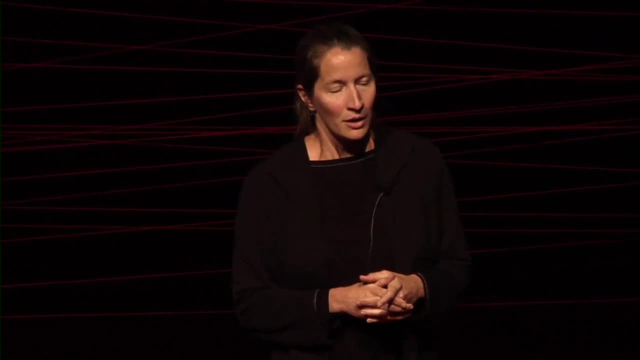 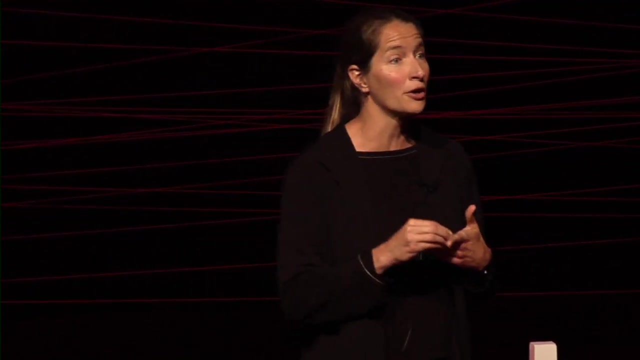 experiments and we have various philosophical games that we use. What we're aiming at when we do that is really threefold. We want to enhance their cognitive skills. so critical thinking They're going to learn. They're going to learn to build an argument. 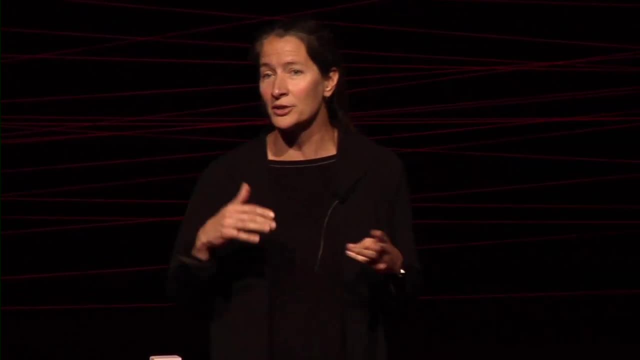 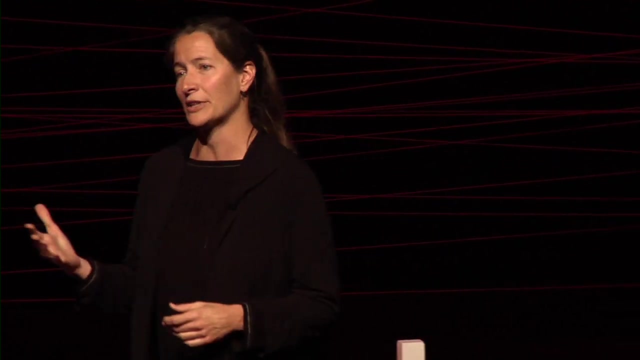 They're going to learn to evaluate an argument using logic. They're going to learn to respond to objections to their position. Those are good skills that are going to do well for them in other kinds of endeavors as well. We want them to think creatively. 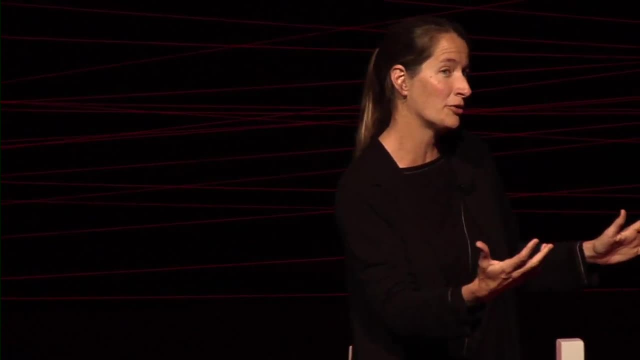 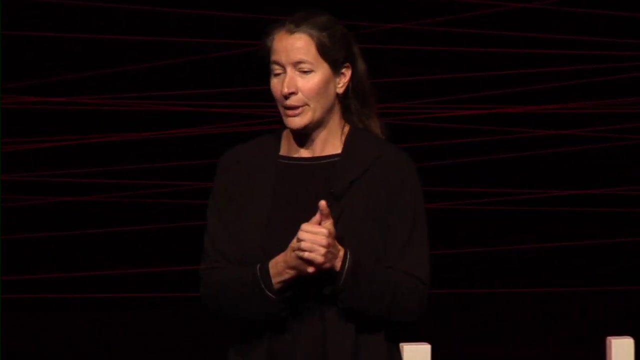 Come up with a counter example. Your friend just made this claim. Can you imagine a counter example or a different alternative? Say what it is and show how it meets that person's claim. We'll also talk about behavioral skills. How can you converse with your peers? 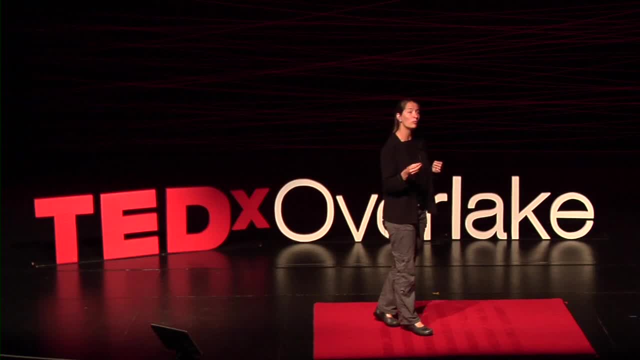 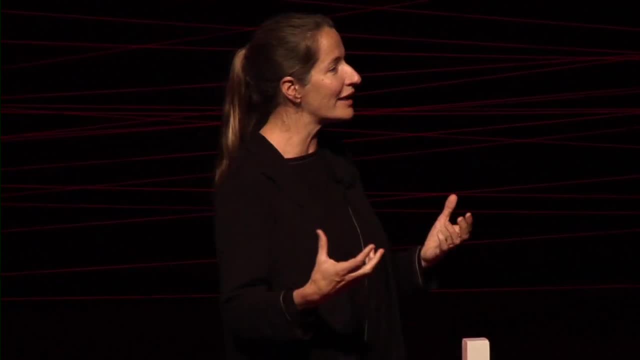 How can you talk to them carefully, take them seriously and disagree with them without fighting or feeling hurt by the disagreement? One of the greatest things is you'll get best friends saying, wow, I never realized I could really disagree with him about something that we both think matters, but it's OK. 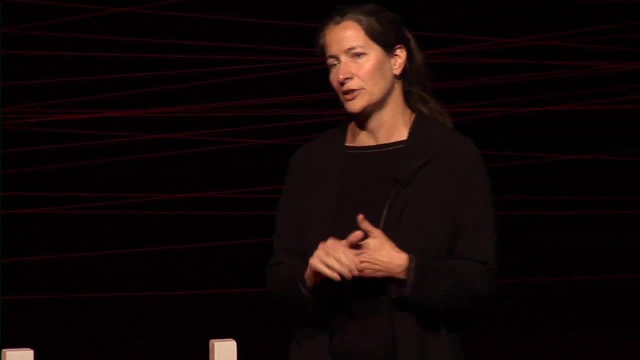 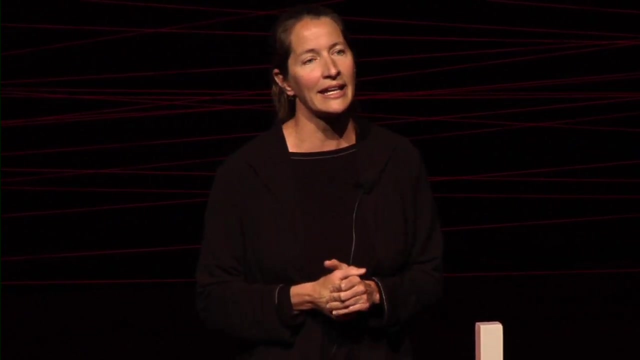 We've figured that out. And then, finally, in addition to the cognitive skills and the behavioral ones, philosophical awareness skills: Knowing what a philosophical question is and knowing that they can answer them. they can work through the data, the difficult questions, and try to figure something out. 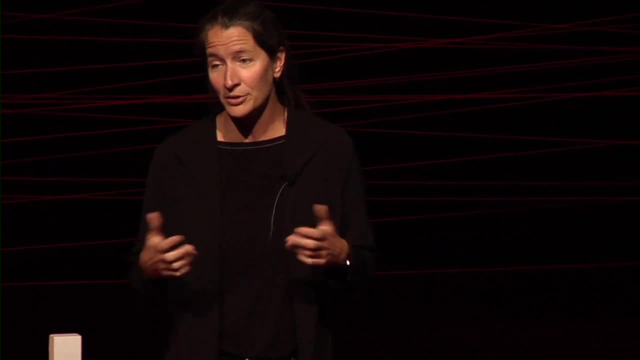 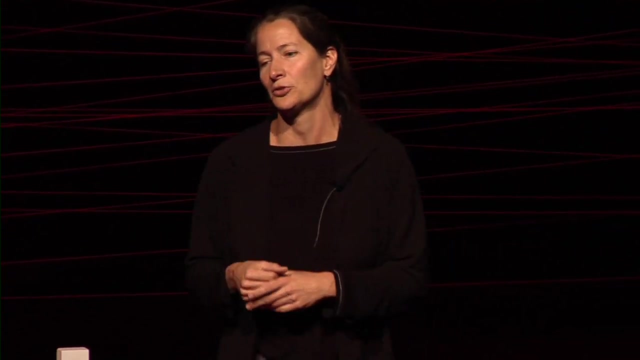 for themselves, I think, is really empowering for them. And what we found, not only in our own work, where kids really enjoy it and love it, but in work done around the world with little pockets of philosophy for children, is that they do better on some of the standardized tests. 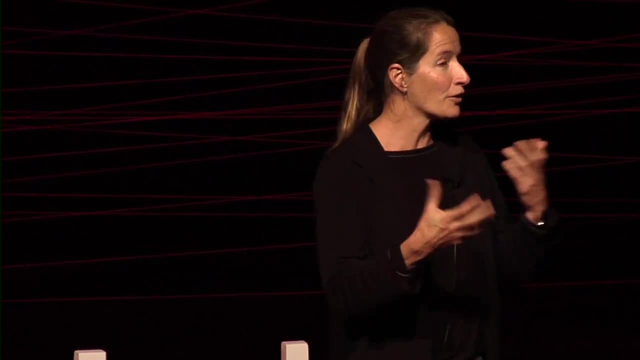 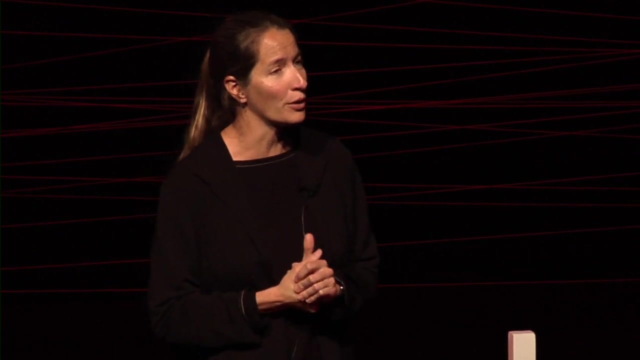 that we have for critical thinking, for language and literacy, for other sorts of things that we are already broadly valuing. And I think, perhaps even more importantly, the students really love it. They are excited by it. It reinvigorates their love of learning. 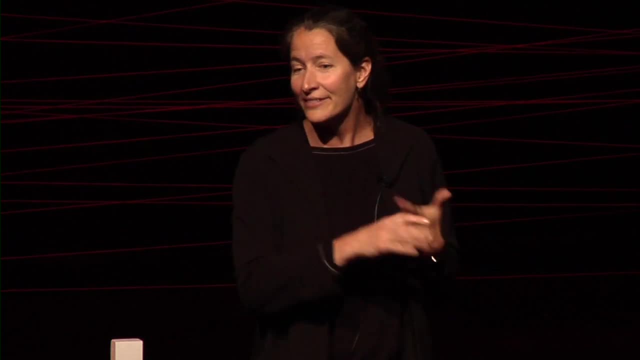 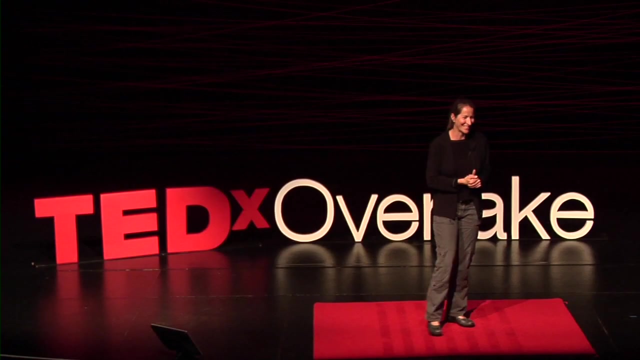 They realize now that these questions matter and that it can be beneficial for them in answering them with their peers, And I think that's what education is all about. That's why we need to do philosophy, Thanks.